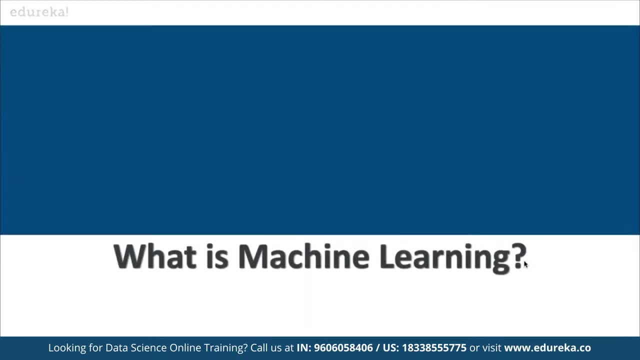 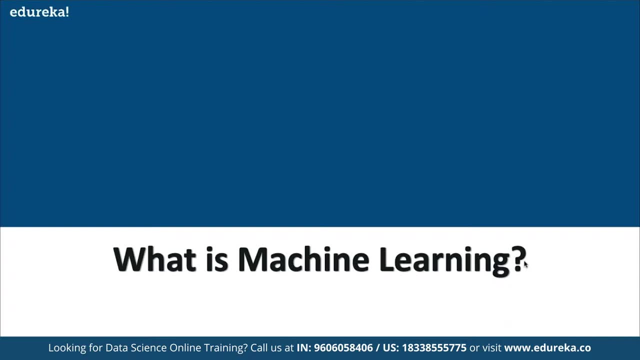 learning. So machine learning is simply making sure that we are going to automate the entire system by using a good amount of data set right. So we can say machine learning is simply the process of feeding a machine enough data to train and predict a possible outcome, using 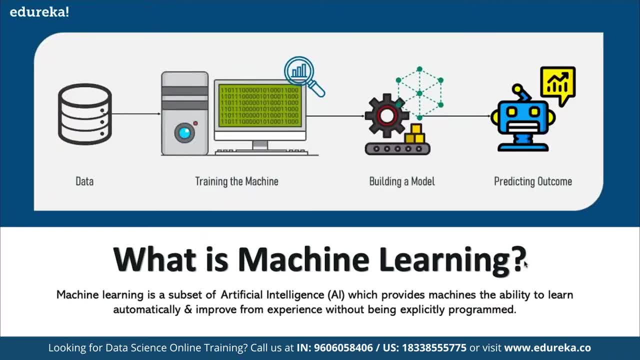 the algorithms with what we have the access to. So, basically, if we use more data set and we can increase the accuracy of the results. And let's say, you may have used Speaker 1. Speaker 2. Speaker 3. multiple predictions made in support before any major match, right? so in this case, let's take an 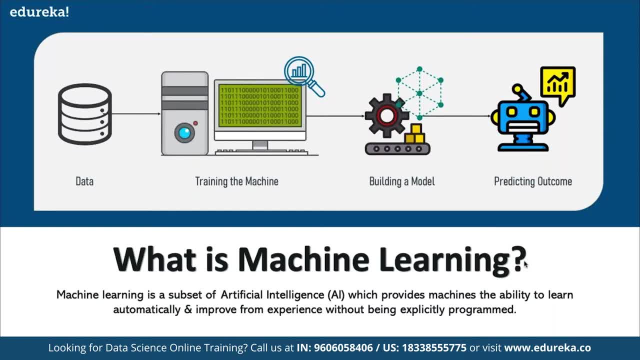 example, for a football penalty session. so the data of previous performances are going to be considered. so let's say the goalkeeper has saved all the penalties to his right in the last 50 penalties he has saved. now this data will be crucial to predicting if he or will will save or he will. 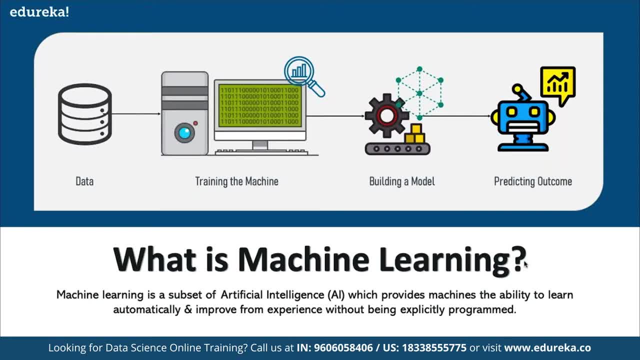 not save the next penalty faces. so there are other factors to consider as well, and another example can be the suggestion that we get while surfing the internet, so the data of our previous choices are processed to give us the most favorable content we are most likely to watch anyhow. 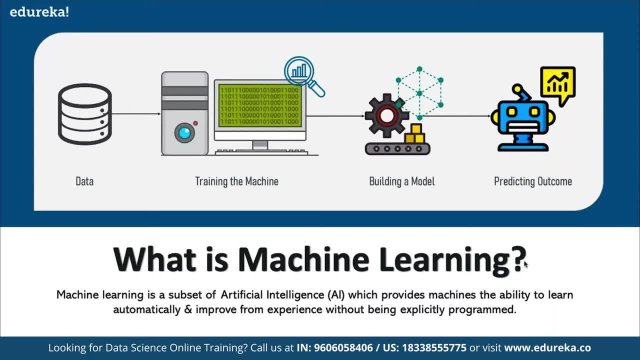 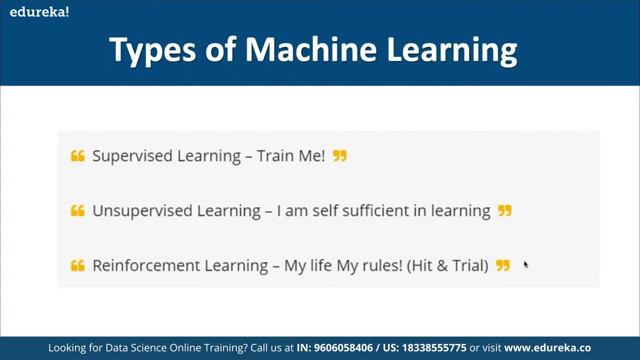 machine learning is just feeding the machine an ample amount of data. there goes a lot of processes, algorithms and decisive factors to get the optimum results all right. so here, basically, we have three main types of machine learning as well, where we have supervised, unsupervised, and then we have reinforcement. 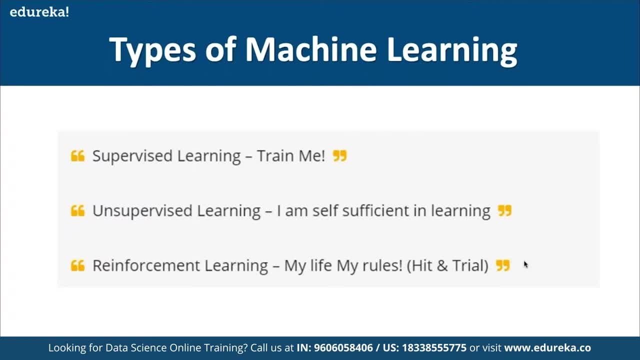 learning so supervised, in simple terms, is: train me. it works on a simple training. we have to train the model, then only it can work. and an unsupervised learning is i'm sufficient. i'm self-sufficient in learning based on their own learning. we are simply going to allow them to have. we're going to allow. 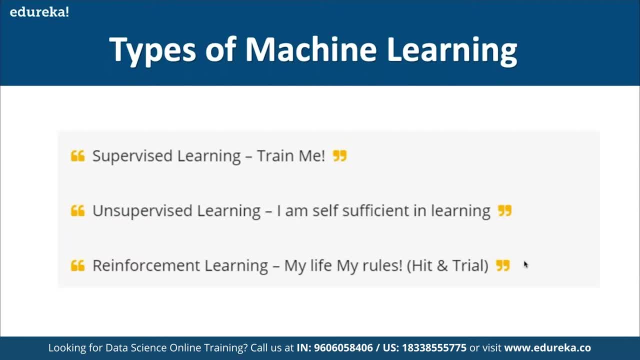 them to have the access as well. so that is what we are going to define for. so, based on their own understanding, they are going to work accordingly. that's how it's going to work, and then we are going to work on reinforcement learning. so reinforcement learning is simply learning on its own, based on 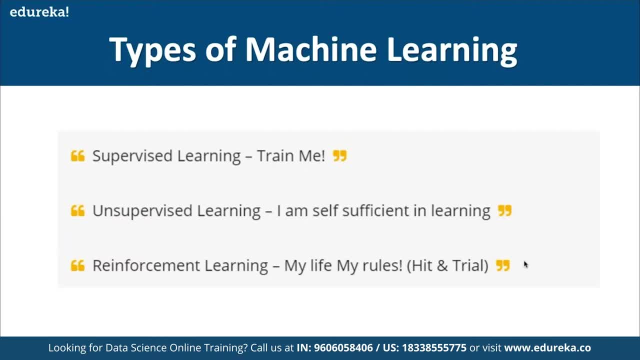 the feedback we simply create. we simply let the system know, okay, if they have done a good job or not, and, based on that only, they simply try to get the best part of the possible output. that's how it works, all right, so, supervisor, in supervised learning, we use multiple label data set to train. 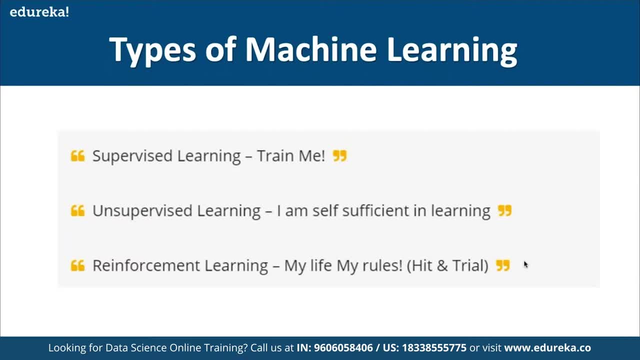 the system and under unsupervised learning. we use unlabeled data set, so the data is sometimes unlabeled or we can say uncategorized, and the machine makes the best, the best possible reference and predictions without any supervision. and then we have reinforcement learning. so reinforcement learning simply ensures: okay, we are simply going to create a system based on the feedback, so the 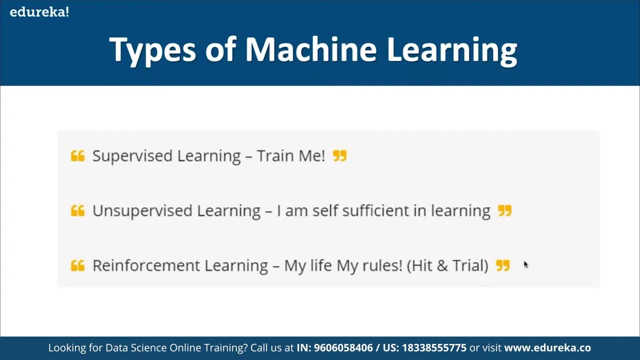 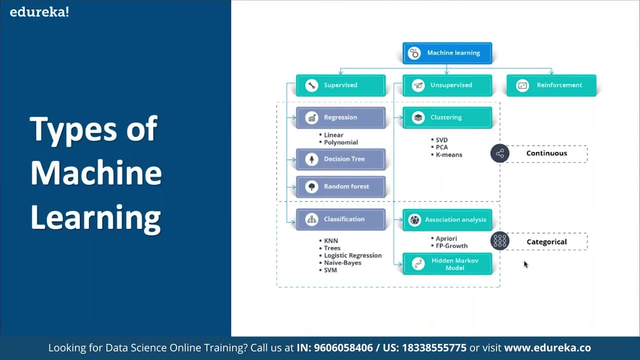 machine needs to establish a systematic pattern of approach in reinforcement learning here. so that's how we discuss again here. we have supervised, again under supervised. we have multiple models that we have regression decision tree, we have reinforcement models. we have different models currently available, whereas in under unsupervised we have multiple models, like we have clustering. we have 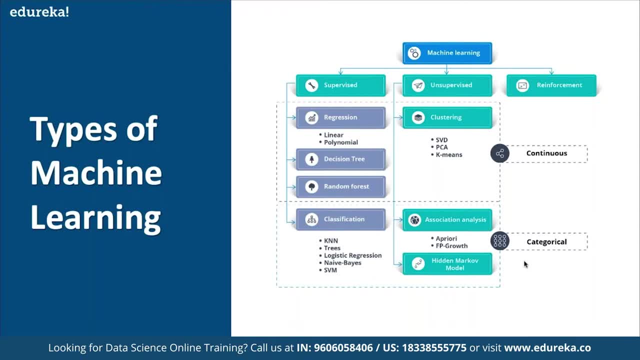 association analysis. we have hidden markup model. so again the knn trees, logistic regression, logistic regression, knife base and svm. they all are types of classification where, if we talk about the a priori fv growth, k means pca, svd. they all are part of unsupervised and again, reinforcement. 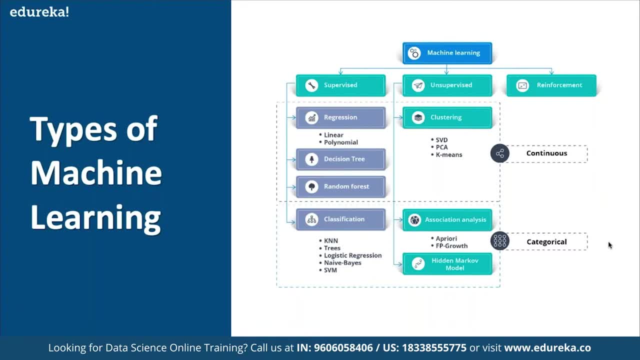 learning is another way that we can define. unsupervised learning is what we are talking about, but under unsupervised training we have information structure, so we are going to talk about that further to design, and then we're also going to discuss in depth knowledge of unsupervised learning and 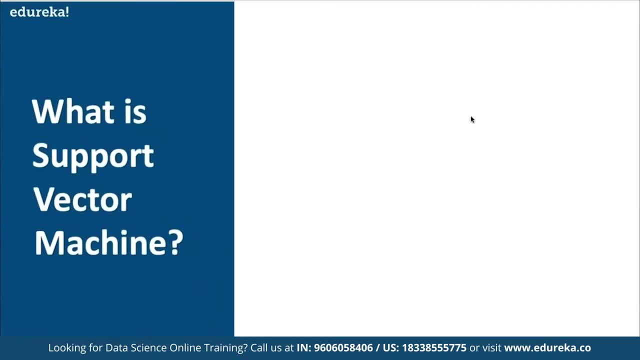 classification data for those two concepts, and we're going to discuss the basic structure of unsupervised learning here, so let me just go ahead and get started. so unsupervised learning is a fairly complex learning machine based on its structure, and its structure is simply based on. 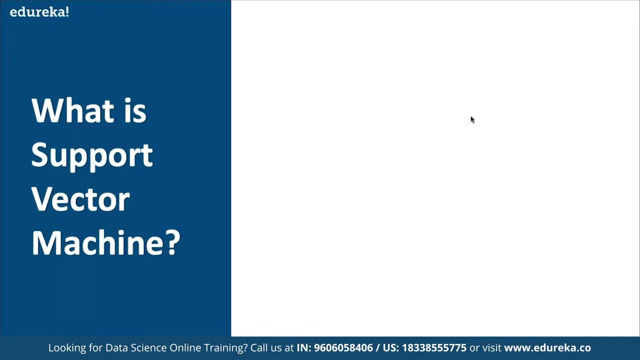 algorithm that has become extremely popular nowadays because of its- you can say- efficient results and, especially for the complicated scenarios, it can deliver it for us as a part of support vector machine. as you can see, I can simply just like a discriminative classifier that is formally designed by: 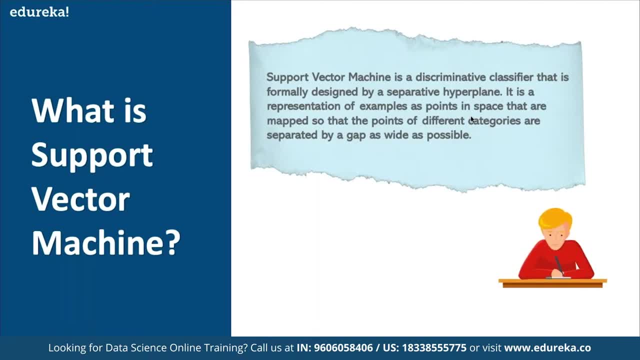 a separative hyperplane itself, and SVM is implemented in a slightly different way than the other machine learning algorithms, so it is capable of performing classification, regression and outlier direction as well, and support vector machine is basically again simply designed by as a separative hyperplane instead, as we discussed. so basically here we can have multiple 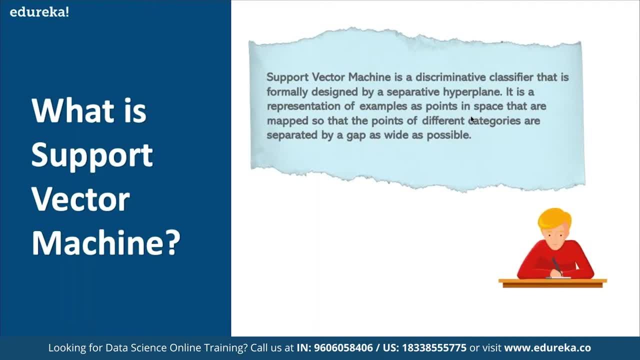 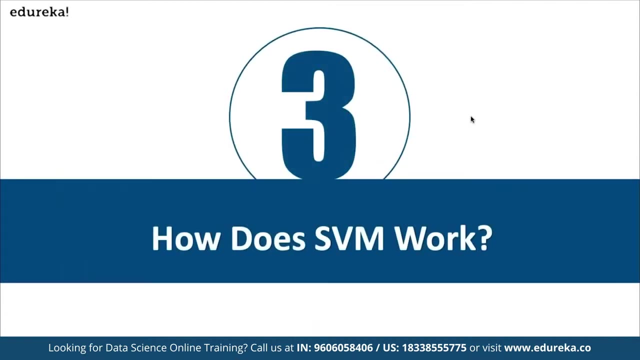 data pointers that can be mapped, so that the points of different categories are going to be separated by a gap, and in addition. so basically, SVM can also perform nonlinear classification. so we'll be talking more about the support vector machine and how exactly support vector machine works as we proceed. 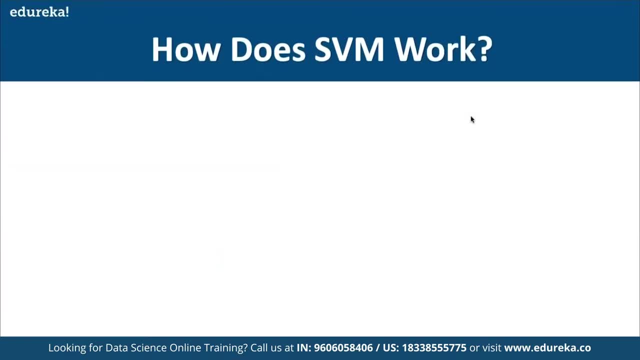 further. but there are multiple advantages of using SVM as well. for example, it is effective in high dimensional spaces, it is effective in cases where the number of dimensions in greater is greater than the number of samples, and it is okay. it simply uses a subset of trading points in decision. 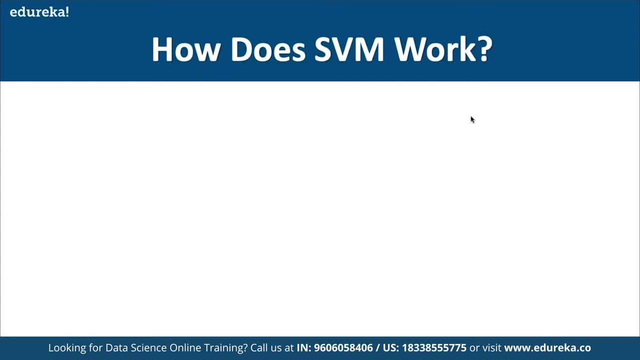 function that makes it memory efficient and it has different kernel functions that can be specified for decision function. that also makes it versus a happy solution, and in the case of SVM it's an intelligent one, as you can see, in this case I can just use a schematic for a Tasks in the data and then I can. 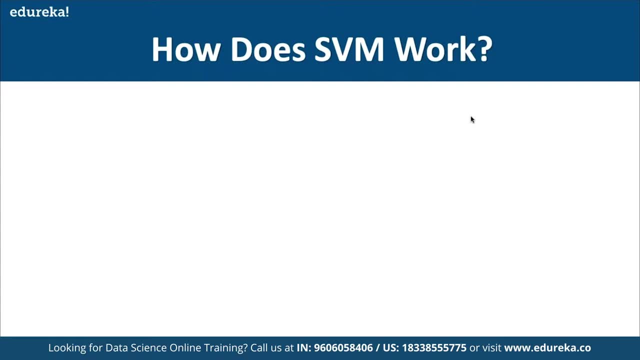 say, I'm going to use a string function to say that SPM is working and SPM is performing correctly. so from here we can have multiple different contexts that are heated and I can easily calculate the amount of time that are needed to create an SVM as well. and same way they also have multiple, we can say downside. 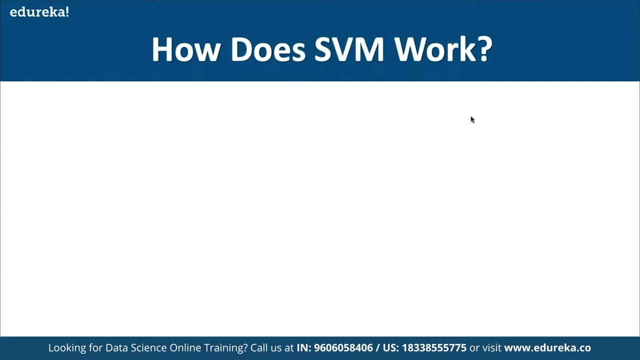 or we can say disadvantages, of using SVM as well. so the number of features is much larger than the number of samples. there we can simply avoid overfitting. main objective of a support vector machine is to segregate their given data in the best possible way, and when the segregation is done, the distance between nearest point is known as the margin. 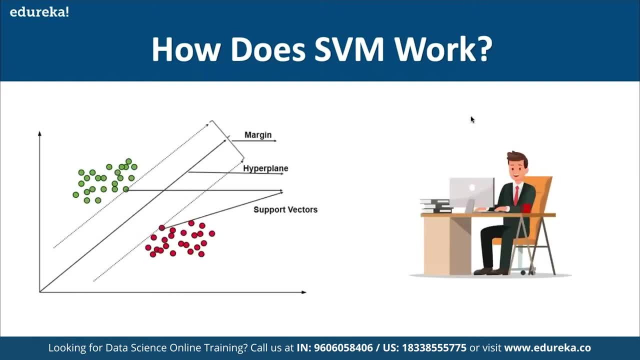 and the approach is set to a hyper, basically hyper, plane with the maximum possible margin in the support vector, as we can see here. that has been right now presented. all right, and now basically here to select the maximum hyper plane. so now here, in the given sets, the support. 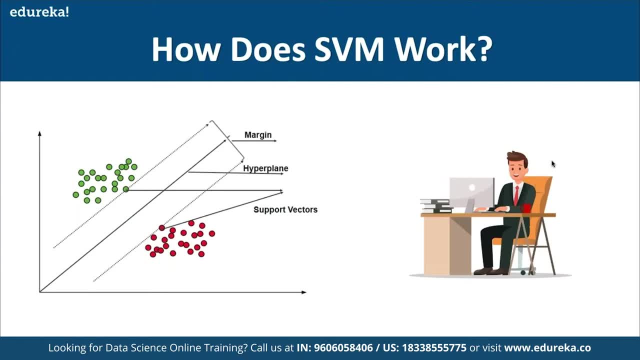 vector machine follows again multiple sets, for example, is simply going to generate the hyperplane which segregates the classic classes in the best possible way, and then we are going to select the right hyperplane with the maximum segregation from either nearest data pointers. so basically, there are different ways of or even on dealing with inseparable or, we can say, non-linear planes as well. 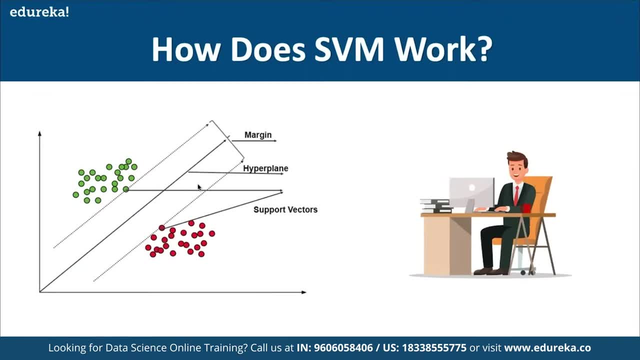 for example, in some cases hyperplanes cannot be very efficient, and in those cases the support vector machine uses a kernel tick for a kernel trick to transform the input into a higher dimensional space, and with this it becomes easier to segregate the pointers. so now let's talk about 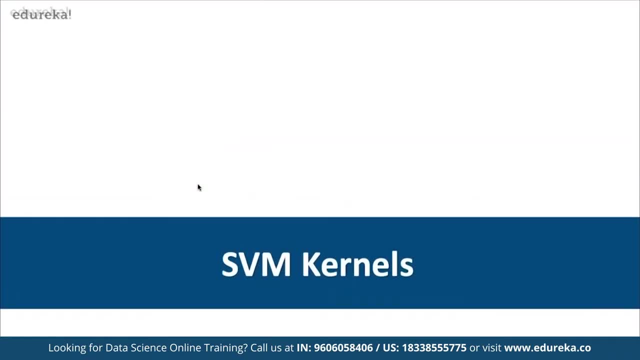 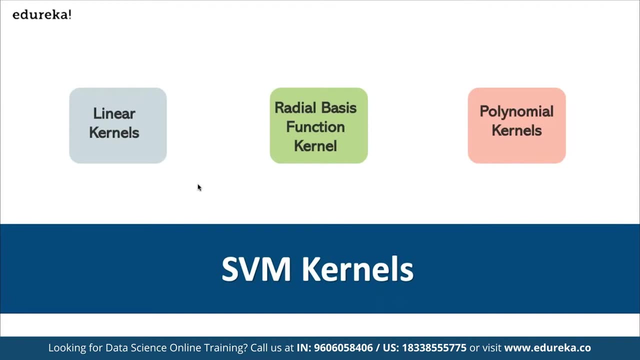 the svm kernels. so basically, svm kernel adds more dimension to a lower dimensional space to make it easier to segregate the data. it converts the inseparable problem to separable problems by adding more dimensions using the kernel trick and a support vector. machine is implemented in practice by a kernel and the kernel trick helps. 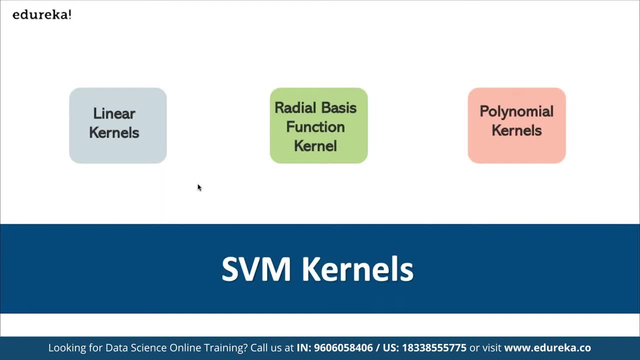 to make more accurate classifier so we can take a look at different kernels in a support vector machine, like we have linear, we have radial base and then we have polynomial kernels as well. first of all, let's talk about the linear kernels, so a linear kernel can be used to as a 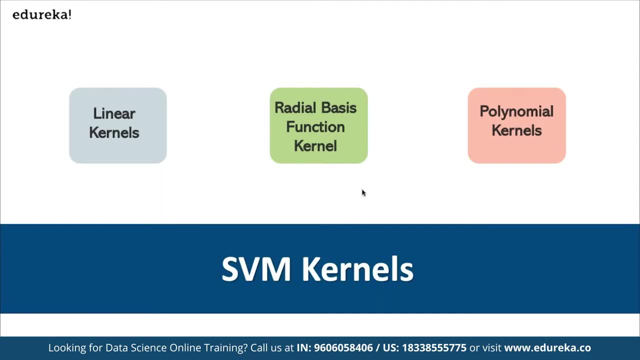 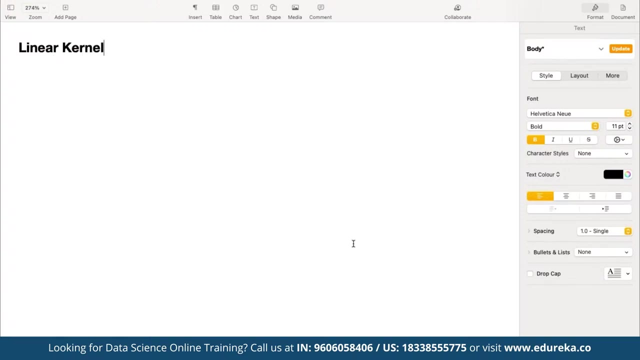 normal dot product between any two given observations. so the product between the two vectors is the sum of multiplication of each pair input values. so we can understand this. so if we talk about the linear kernel, so basically, as we as we discussed, linear color can be used as: 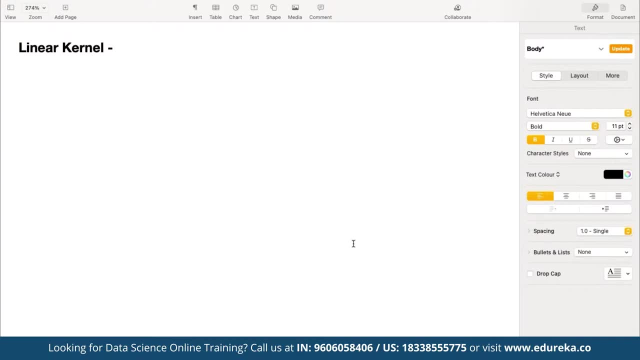 normal dot product between any two given observations, for example, here we can define this one as opposed to zero, and it can be added to sum of, let's suppose, multiplied by x, x, i. all right, so as we discussed again here it is going to be, the product between two vectors is the sum of multiplication of each. 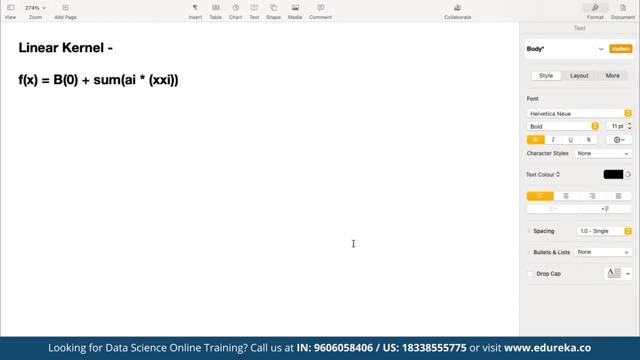 pair of input values as a part of simple linear kernel equation. and then we have polynomial. so this one is for linear, then we have for polynomial kernel. so polynomial kernel is what polynomial kernel is like, a it's rather generalized form of the linear control and again it can distinguish curved or non-linear input space. 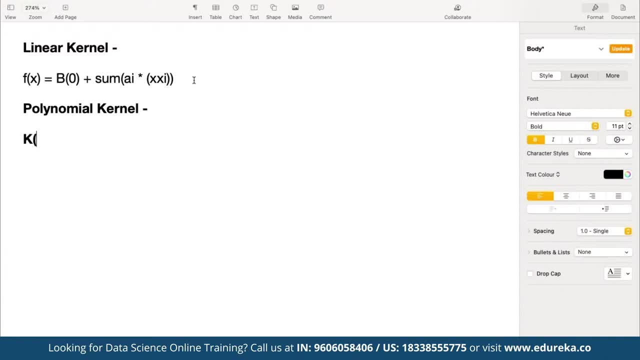 so for example, here we can refer this as opposed as k, and then we can define multiple pointers, i suppose x1, x2, and then we can simply add this to a plus. now, here we have defined, suppose x1, and again all of the defined here: x1, t, and then x1, for again this value for x2, here for x2 and again the entire one. 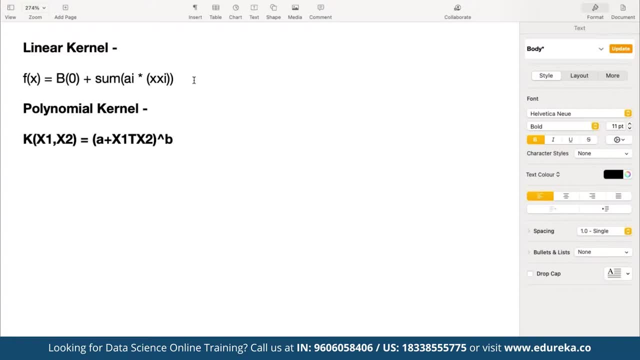 has to be raised to power b itself. so next we, after polynomial, we are going to have- we also have radius space. so here, after polynomial, we have the radial basis function kernel. so in terms of radial basis function kernel, so here the radial basis function kernel is commonly used in the svm classification and it can map the space in. 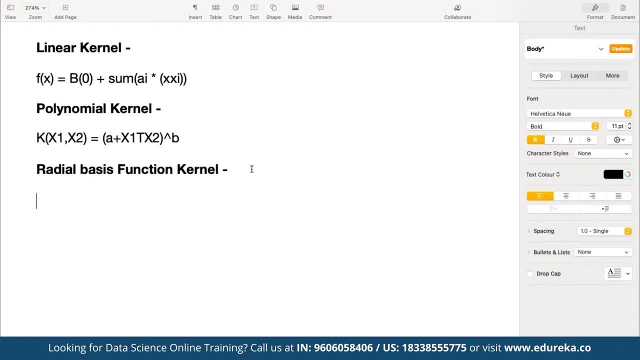 infinite dimensions. so basically, if we talk about the actual dimensions here, so here we can represent it as opposed, the value of k, x1, and again for x2, and here we can find the exponent where x is going to be supposed for minus 4, again the gamma value, and 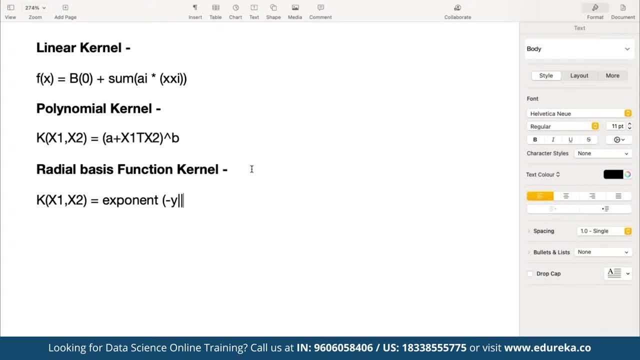 let's say we represent this as y, and then we can define this for x1 minus. this is going to be x2, and then it has to be raised to power 2.. so basically, x1 minus x2 is simply going to be the euclidean distance between the x1 and x2. 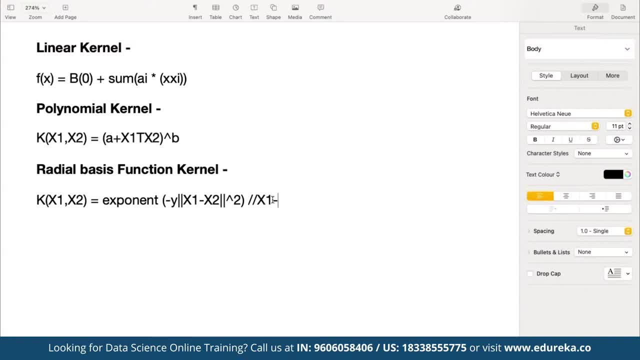 now is euclidean, so here on the x1, so we can say: x1 minus x2 is euclidean distance, is the euclidean distance between x1 and x2, here and where, if we talk about here, if we talk about the current component for b, so here we can say b as well, b is, b is the. 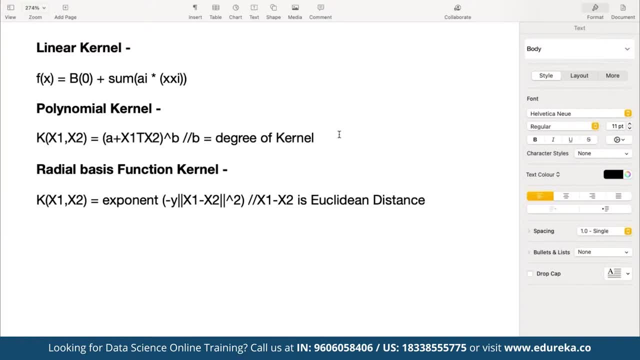 degree of kernel, in case you don't have, in case you don't have the knowledge of the kernel. so we can knowledge of offered yet and then a is going to be. or we can say a is what is the constant sum is the constant term that we have. so here we have linear polynomial and then we have radial basis. 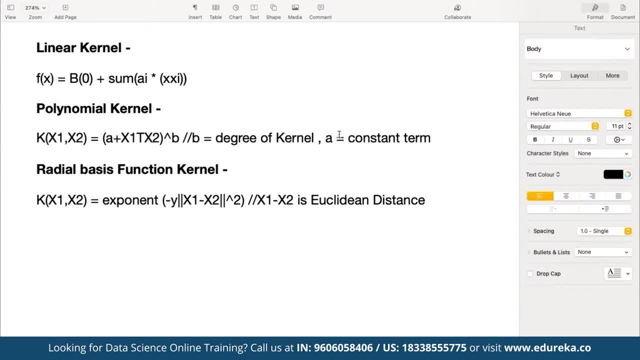 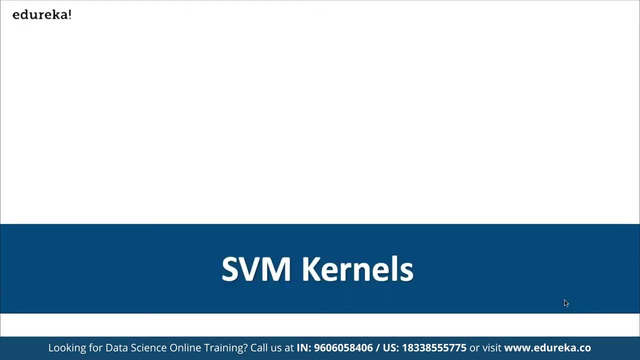 function, so there are multiple use cases. so before we proceed further, so there are multiple use cases. of the serial base conver, i can say component as well. so here we can use it for the phase selection for text and hypertext categorization. here we use it for the classification of images. 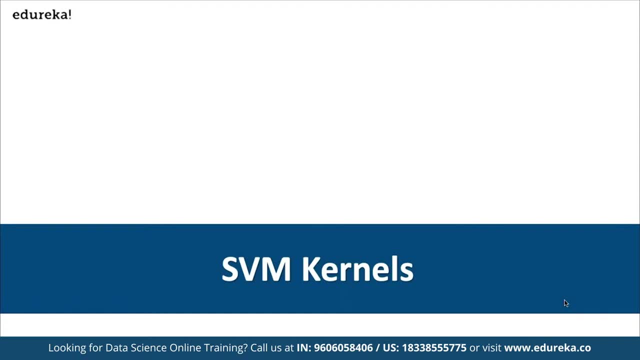 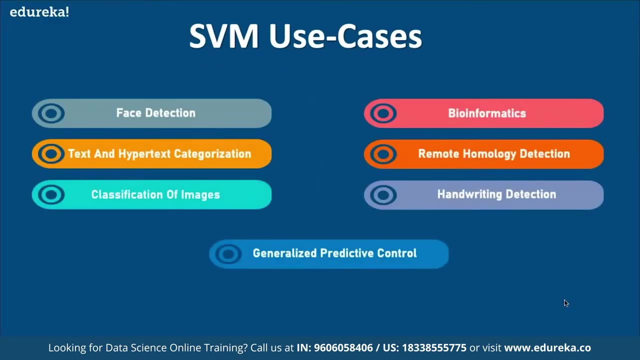 for bioinformatics, for protein fold and remote homology detection as well. we can use it for different use cases and we can also use for again having a prediction control as well, as we discuss in svm. so there are multiple use cases for phase selection for bioinformatics. 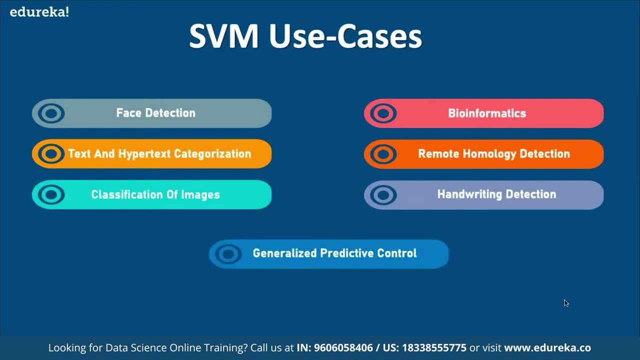 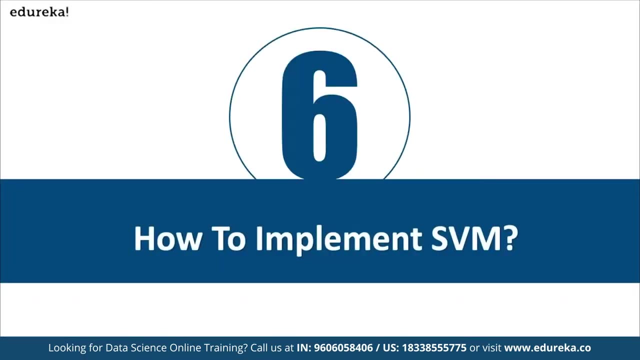 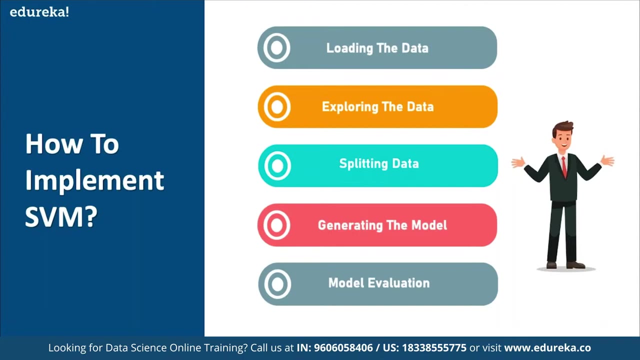 for text and hypertext categorization, for remote homology. these are different use cases are currently available here. so now in terms of how to implement svm. so first of all, we have to load the data, we have to explore the data, we have to split the data, and then we also have to generate the model, and then we have to evaluate the model as 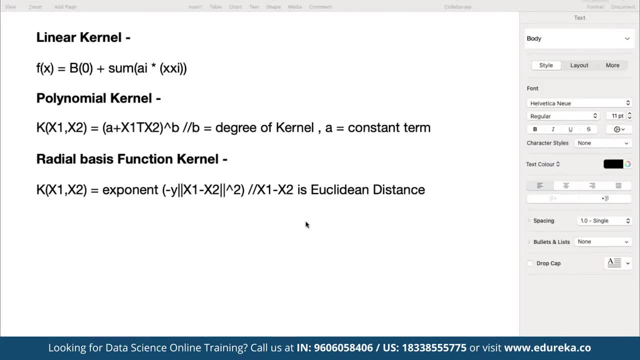 well, as we have discussed again, in case we haven't confused. so, linear is simply going to be the dot product between the any two given observations itself. and here we define two: here the product is going to be the dot product, and here we define two: here the product is going to be the dot product. 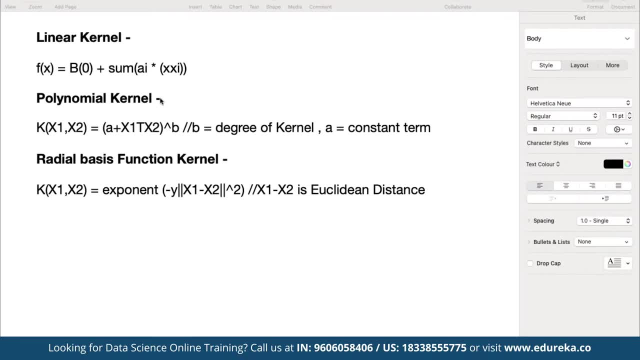 between two different vectors. it's simply going to be the sum of multiplication of each pair and then under polynomial. so basically here we can distinguish curved or non-linear input space where we have defined the k1 as x1, x2 for where a is, where a is simply going to be a constant term. 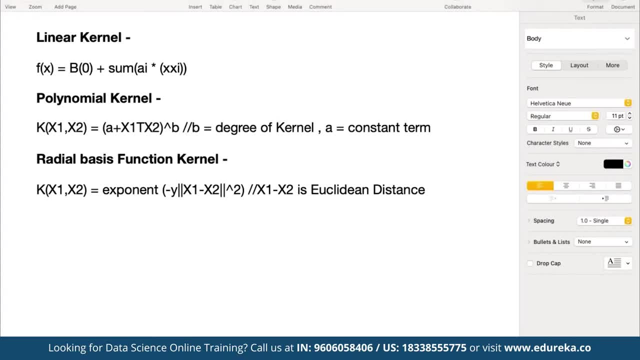 and b the power to which we have increases. so b is simply going to be the degree of penalty are going to make use of and then under radial basis, as we discussed. it is commonly used in classification and can map the space in infinite dimensions as well, where x1 minus x2 is simply going to be the euclidean distance sensor, as we can say this. 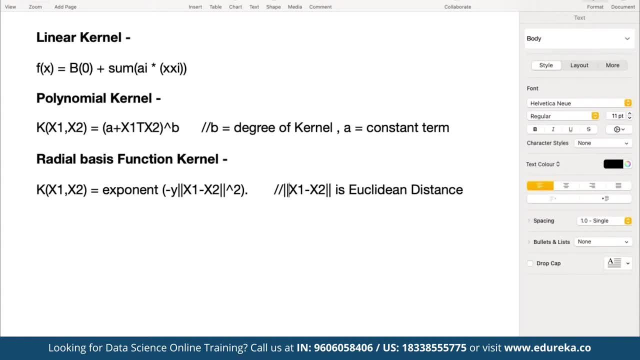 one that we define here. x1 minus x2 here is simply going to be the euclidean distance here. all right, so let's do one thing: let's open up fai charm community here so we can start by simply loading the dataset and then working on top of it so we can use any id we 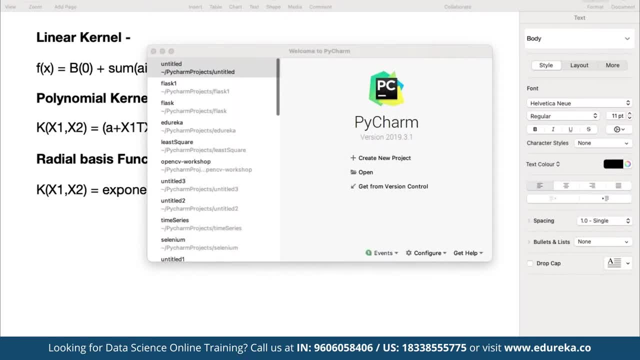 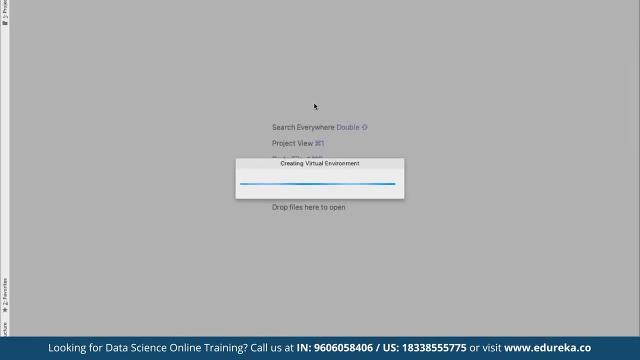 any python id to get started. we can use anything. so let's do one thing. let's create a new project, let's say we name it as svm. so in case you don't have the access to svm as of now, so you can go ahead and download the community version. so this is going to give you the access to pycharm, or 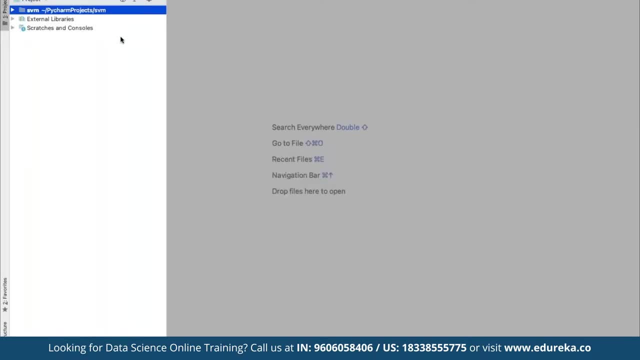 we can use any other id as well, if required. all right, so here, once we have the project here, we can simply go ahead and create a new file altogether. so let's name it as our demo file. so first of all, we are going to work from the skln library, so here we can use from skln. 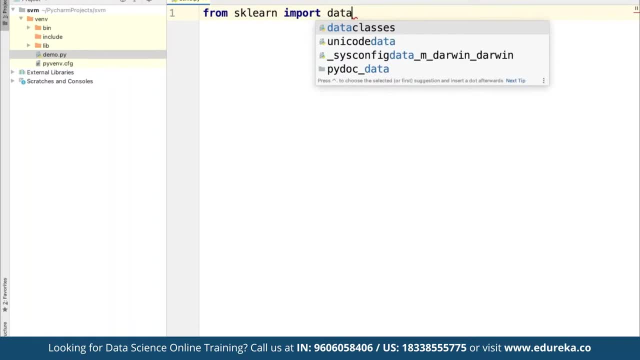 we are going to import the data set. so they they are some sample data set available under skln library itself. so here we can define the cancer data set already available under skln and here we can use data sets dot load and then we are simply going to load supports for. 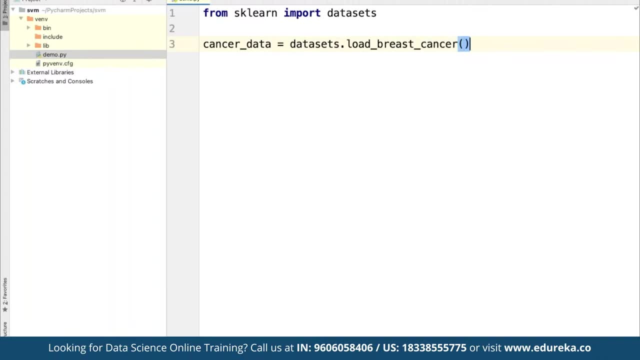 breast cancer, we can load this current data set already available. and now, if we want to simply print the current data set that we can, that we have currently imported, so here we can define cancer data, dot data and again we only want to print the five first rows available in that. 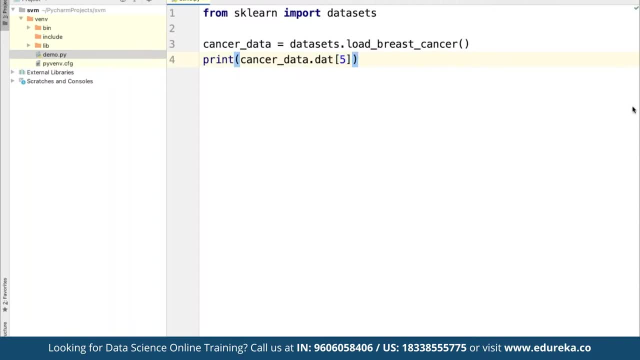 so here we can define these statements here. so we have, we are going to use a sample data set available and whenever we are going to work on any project, in case they are now, in case the data set is not available, then we can go ahead and simply install more libraries by simply. 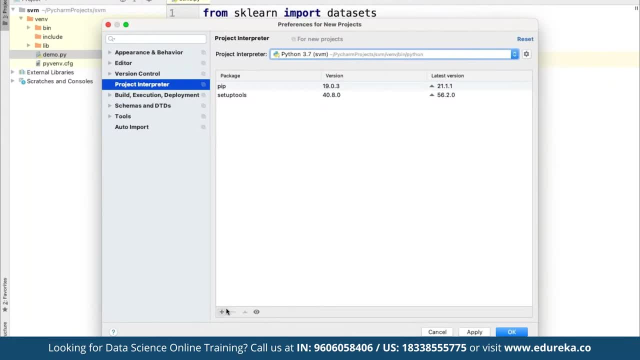 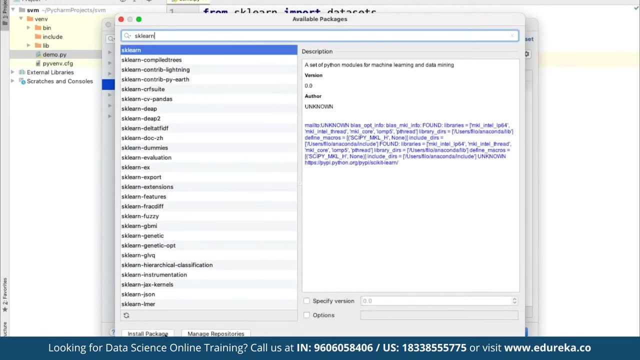 choosing the current data set and then here we can go ahead and click on add and from here we can search for any library that is that we may that may be missing. for example, here we are going to work on sklan, so we have to make sure that we do import skl, because without skl library 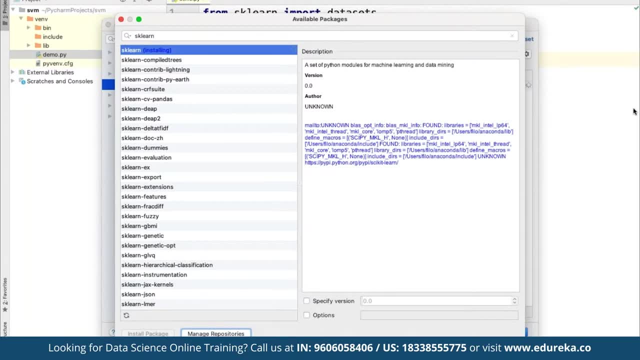 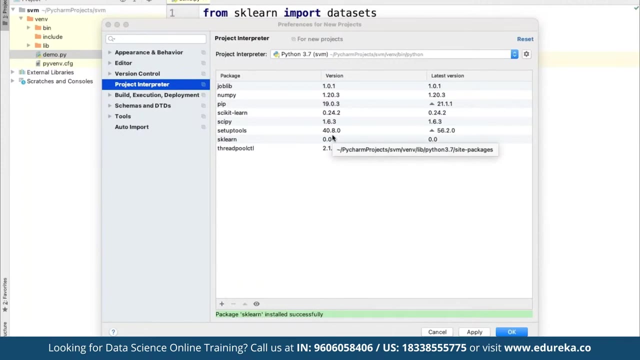 we will not be able to work on the svm here, so here we are simply going to work on the sample data set. all right, so as you can see, now skln has been installed. so again, this is a. this is a packet that we're going to work with, so here we can close it if we want to work on. 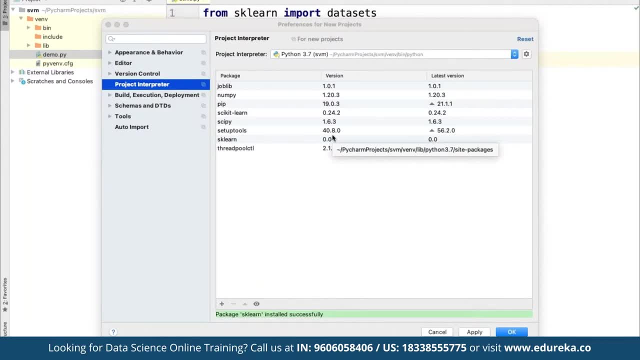 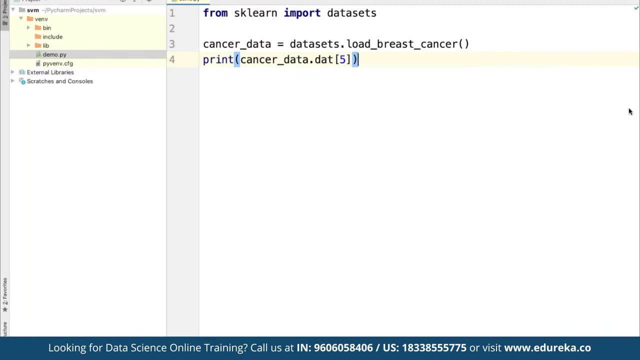 the other components, we can search for any library and then we can have it installed. all right, so now we can click on apply and then, once we now, because we've already created this one, we can go ahead and click on apply. and if we don't have the library, 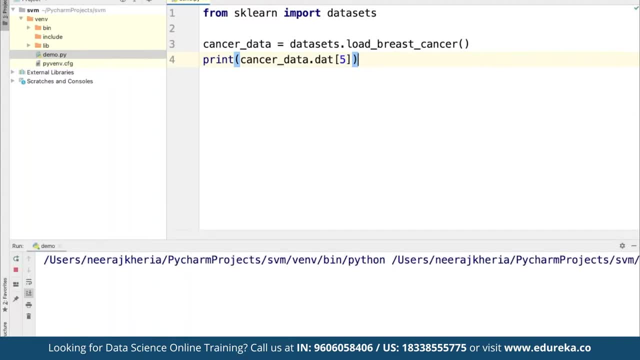 installed and then if we try to run this up, it will simply go to throw us an error and, as you can see, currently this is going to update the package and then from there it is simply going to load the breast cancer data set which is available as an inbuilt sample in sklan. so, 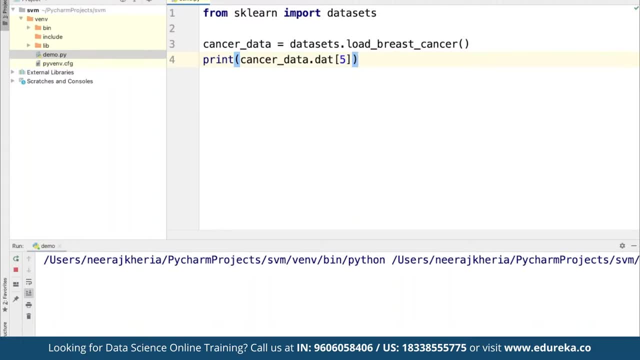 it is simply going to get connected to the server and then from there it is going to be going to pull the load- the breast cancer leader set- and then it will simply go to print the first five rows. So it may take a while, depending upon how which there is that we have imported. 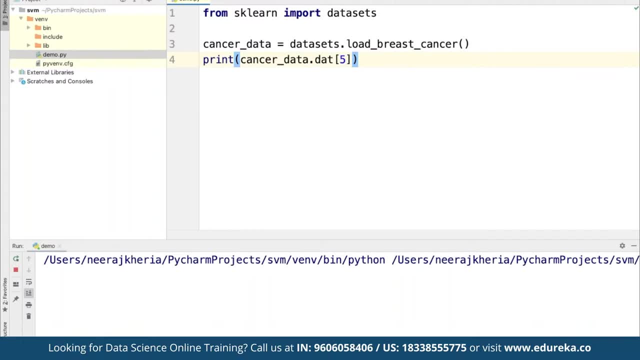 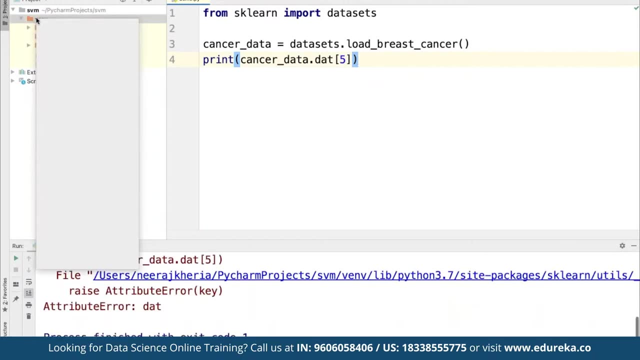 So before we perform any calculation, let me just show you how static this looks like again. in the meantime, this is getting pulled here, So we can simply go ahead and create a new file. It has been timed out Because of memory error. 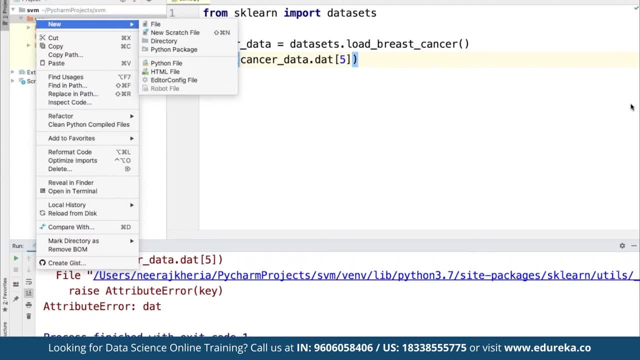 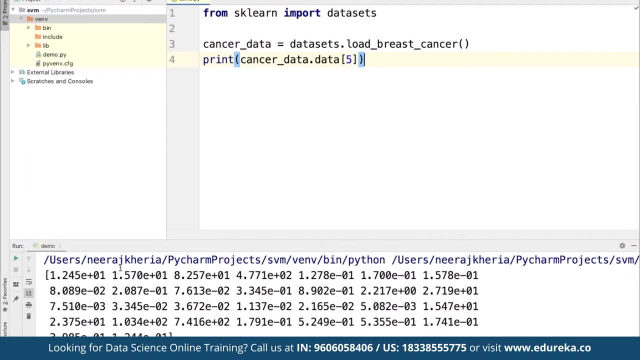 Okay, we define, we misspell data. It has to be data. It's a bit only to simply going to face the different there. So, as you can see, here now we have the first five rows in terms of this breast cancer data, which. 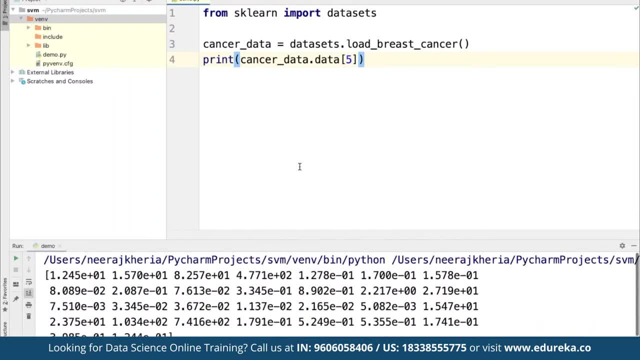 has been pulled automatically from sk-9, as you can see here. right So now we are going to here, we have defined the data set, right So now, if we are going to simply split the data, right So we are simply going to divide the data into trading set and the test set to get accurate results. 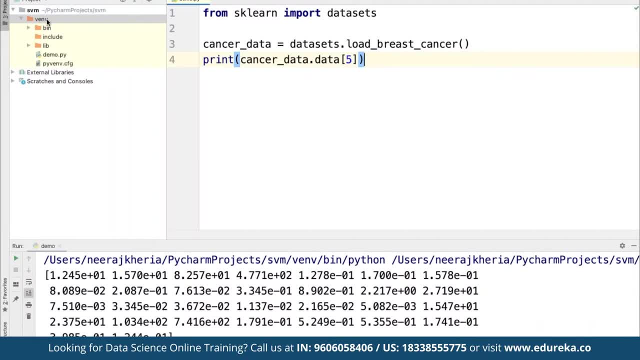 and after this We We will split the data using the train test split function. So here we are going to need three parameters, like in the sample that we have that we are going to see. So from here we are going to load the current data set. 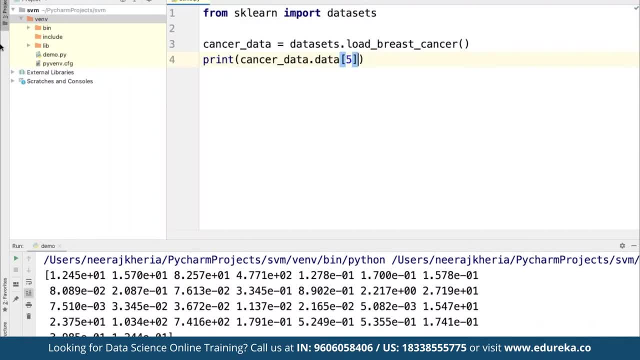 So for example now here, not just to avoid confusion for your- so we can create a new file. Let's say we define some as post Emma to. so here we can define from sklearn. So first of all we define from sklearn library, from sklearn. 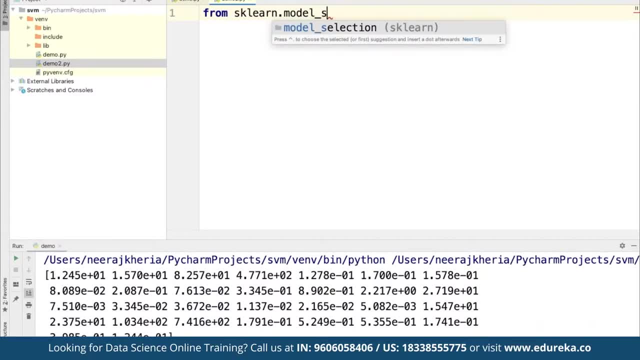 dot model and here we can define model selection. So here we are going to import train test split. as we discussed, We are going to split it and then we can define from cancer data that we are going to import. So here we are going to find data set, dot load rest cancer, which is already available. 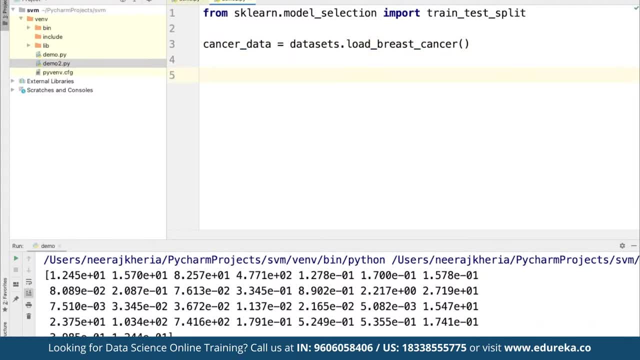 And then we are simply going to define the models in terms of: suppose here We define extreme, And then we can find X split. We get a plan for X test, and then we get to find same thing for Y train For Y test. 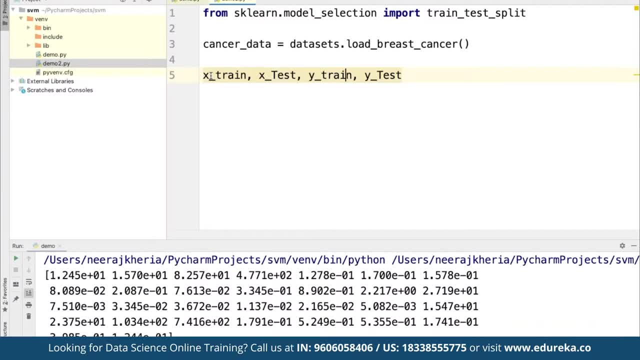 X train X test. Y train Y test. So here we are going to define this from the same train test Split that we have going to import and then here we are going to divide them under, from the cancer data and the data which has been imported here. 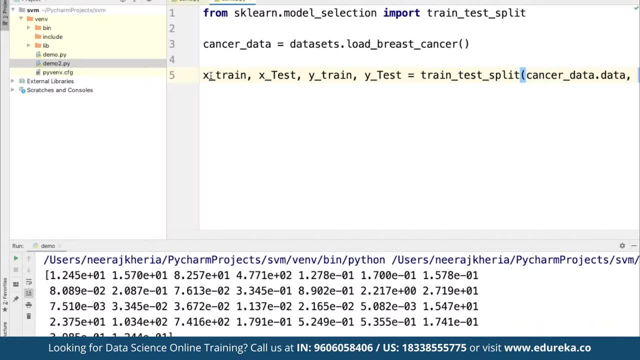 And then we are going to define this for cancer data target. So say, here we can find this for cancer data dot target And then we can define the test size. here We get to find the test size. Suppose we want to keep the test size opposed as four. 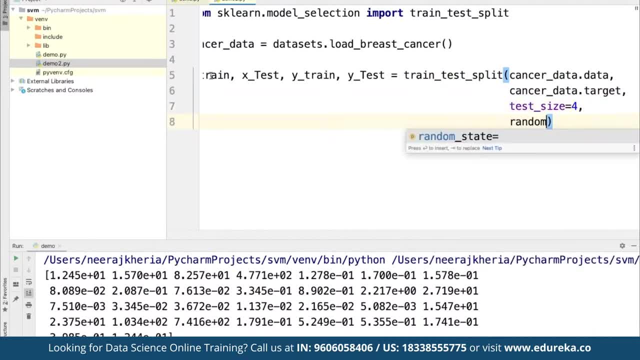 This test has as four and then we're going to find random state. We can find random state, Suppose we don't like anything that we want to have. So here we are simply going to split the data set with the given in the extreme X or X test and the Y train and Y test here. 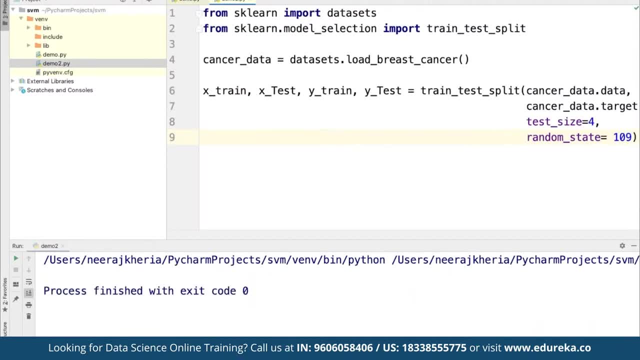 So here the entire set is simply going to be split. So, as you can see, now that we have split the entire data set, So now we are going to generate the model as well. So what we can do. So now here we are going to change. we can say: generate the bottle and for that we can import on the library. 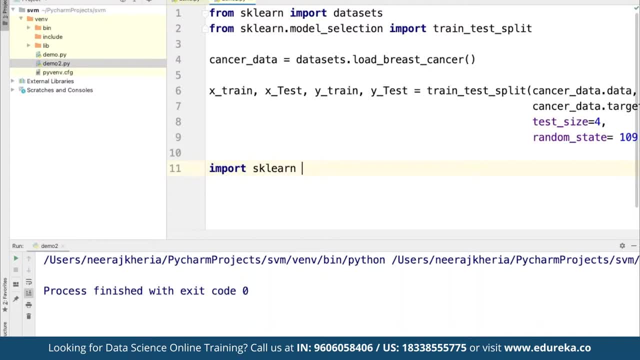 For example, here we can import, let's say, a scalar, and from escalon We are going to import the SVM. So here we are going to create the library. So here we could create a classifier here. So first of all we're going to find classifier as opposed SVM, dot, SVC. 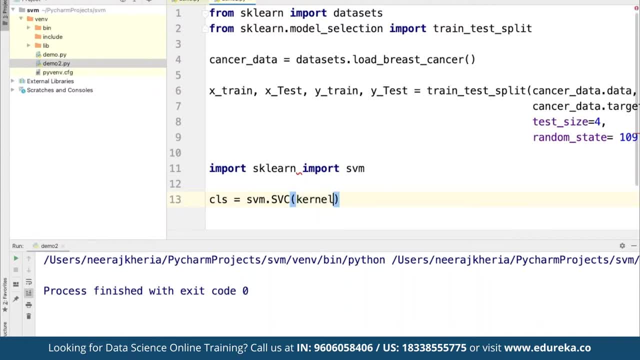 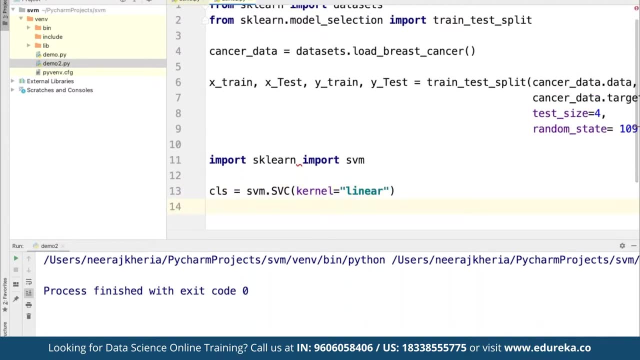 And here we can find the classifier Kernel. here We can find the kernel as opposed linear. What do we want to use? We can find that and then we are going to train the model. So you can see, we are simply going to not train model. 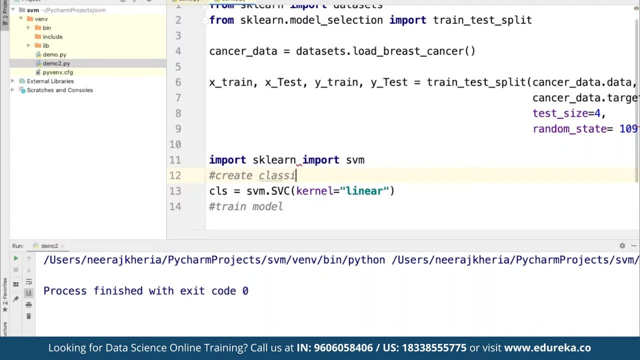 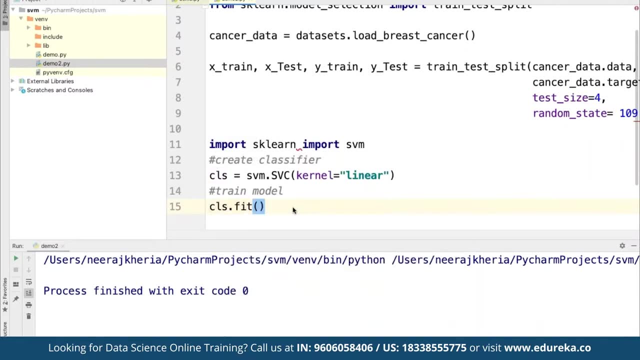 So here we have create classifier and now we are going to train the models. So for training one we can define class dot fit, and then we can define this value as extreme that we have already imported and then we can define for Y train that have we have already before the split on, and then simply we are going to have a prediction done. 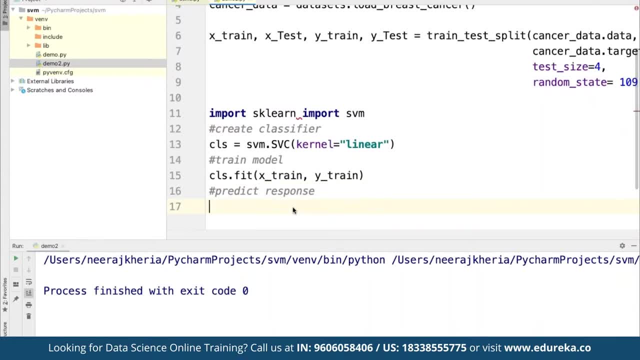 So here we can define predict response and for getting response We can define prediction as class dot predict, and for this we are going to make use of X test that we have already defined. We define for extreme and for Y train and then for prediction. 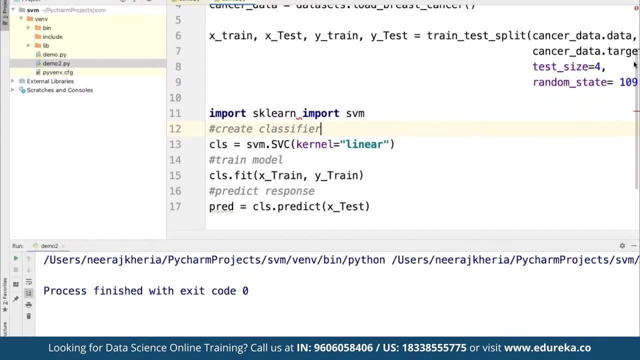 We are simply going to do that. on the text on The X underscore test is that we already have to find? That depends upon type of data that we have. So that totally depends upon the type of data We are going to simply import. 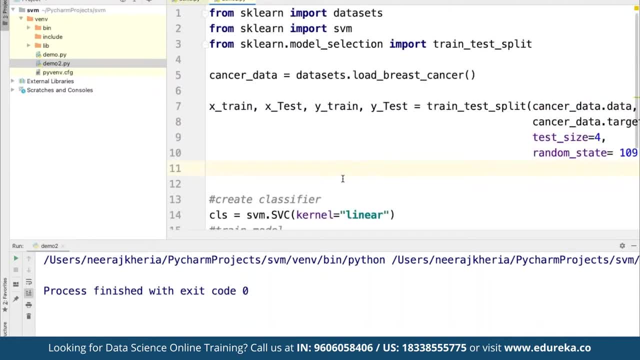 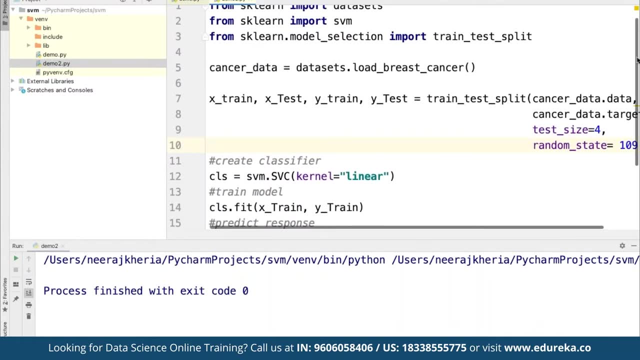 And let's move this import from the end up here. So you have to find this in the top section. So from a skill, and we are simply going to import the estimate that we had to find on it. And now we had to find a classifier. 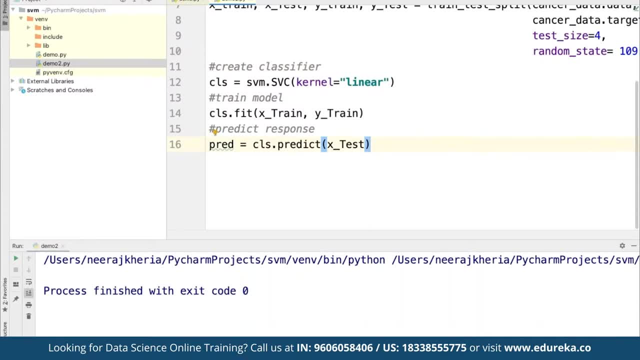 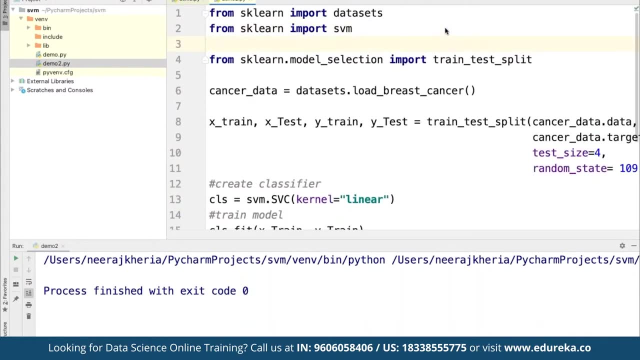 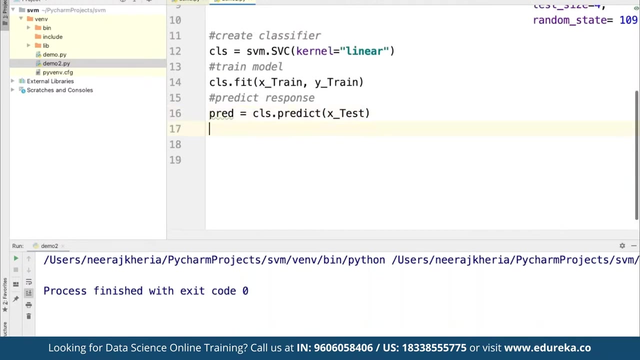 Now we are going to evaluate the model and for evaluating the model We can simply go ahead And define. So here from a skill, and we can also import other components as well from a skill, and we are also going to import metrics. So here we are also going to import metric and by using back your accuracy metric for getting the accuracy. 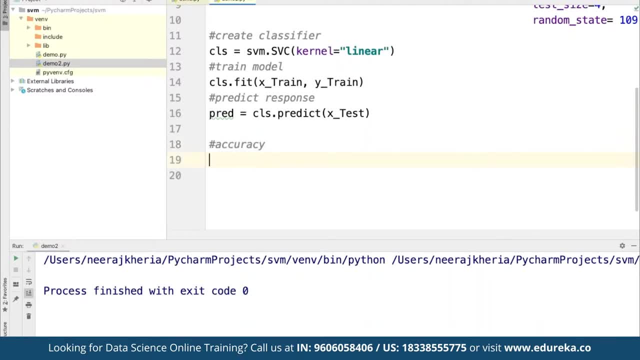 We can find for getting the accuracy We are going to define. We are simply going to print The accuracy of the prediction here and, for accuracy, We are simply going to define metrics, which is again Available under the matrix that we have. 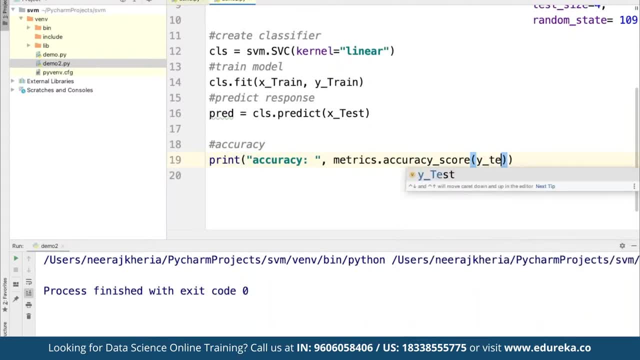 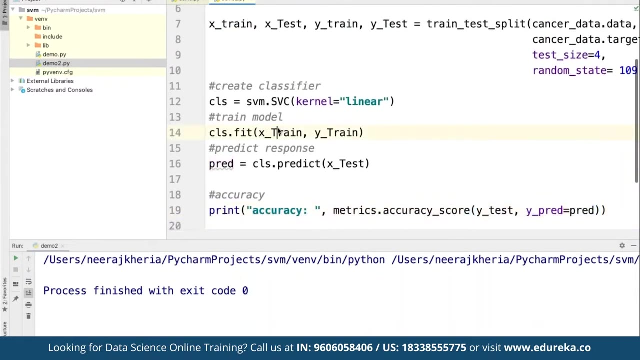 We have accuracy score and then from here We are simply going to find why test and we are going to find us before Why prediction as well, that we have defined. I think we have used why test, we have used up our case, But for we have used, let's do one thing. 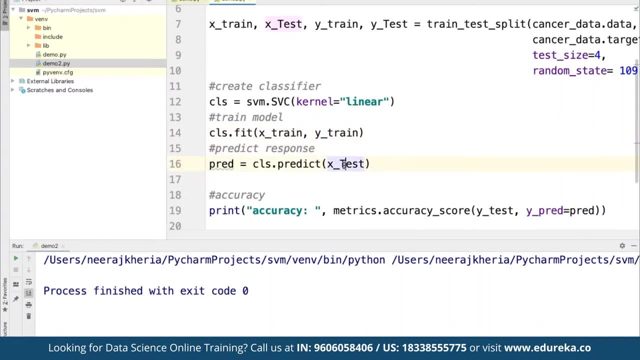 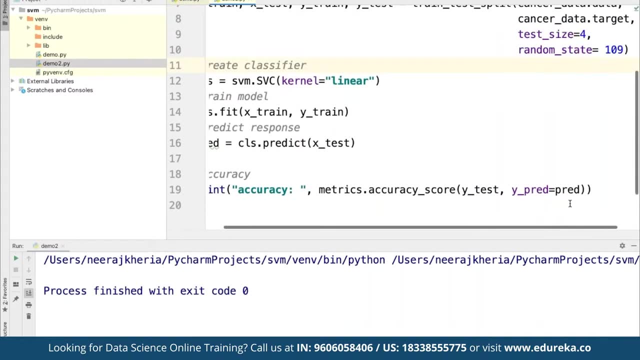 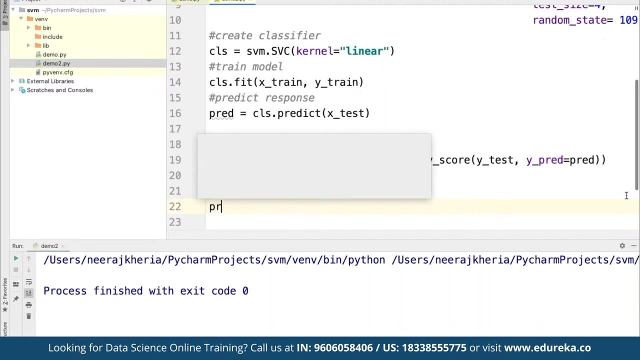 Let's use small is for everything, just to word confusion as a fun says: test Again and test again. So you have a white test and then you depend here. We define it for production and then for finding the precision score. For finding precision we can simply print: 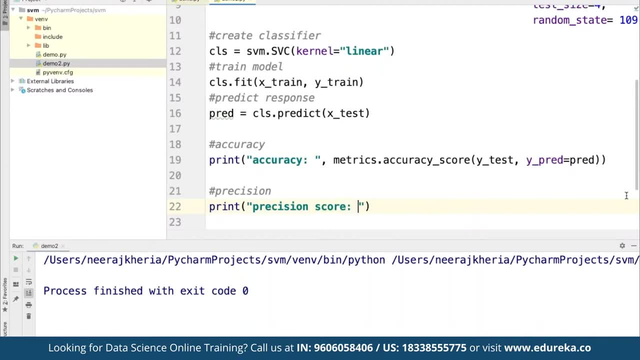 Another statement as precision score, And in here we can again make use of metrics, and for metrics We can define the precision Score itself. So here we can define Precision underscore score, And in here for precision score, We are going to make use of y test. 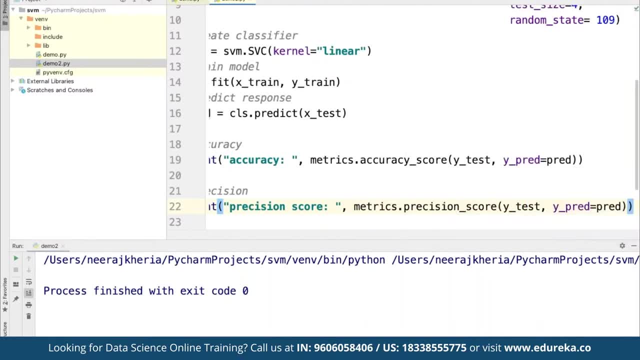 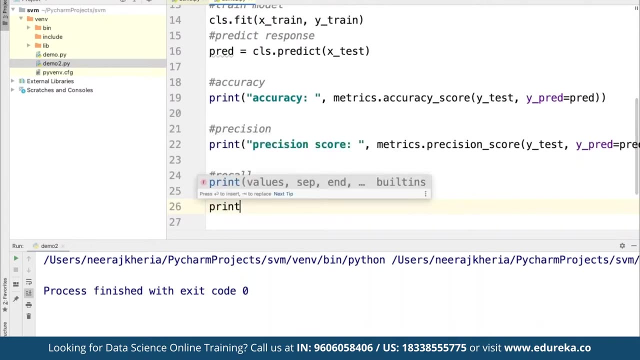 And then we are going to make use of y prediction, All right. and then at the end, if you are simply going to recall the score and we are simply going to report, So here we can find for recall, We can print other statement. 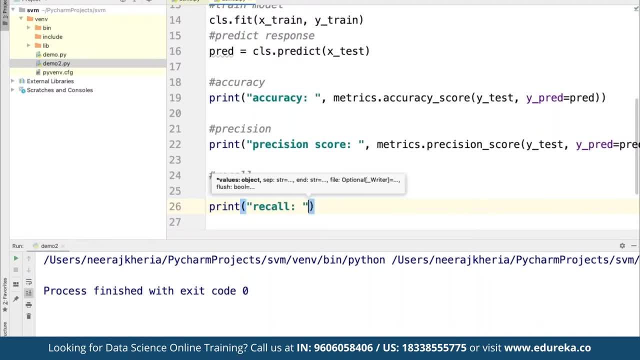 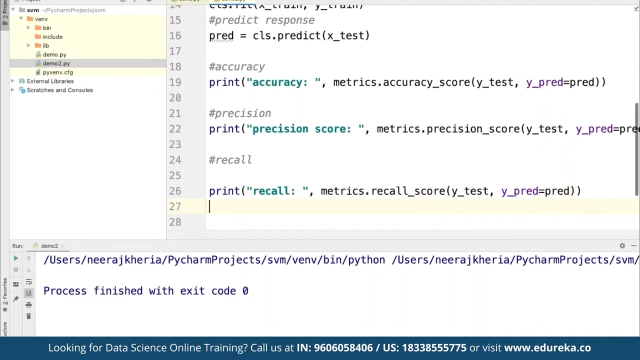 For recall, we can define this one as recall And here from save metrics, dot recall Score and for here we can find Why test And why Prediction for the prediction that we are going to define. And then if you want to print all the metrics, so here we can find print metrics. 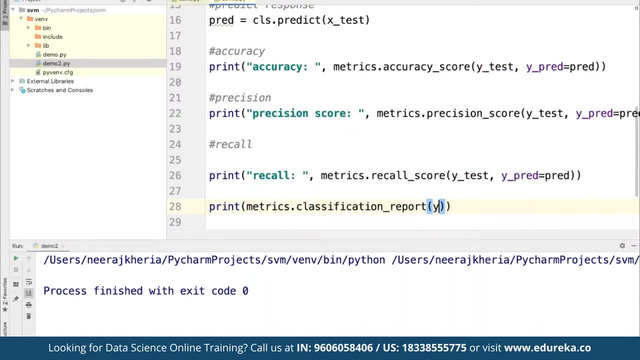 Dot classification report, And for that we are going to make use of y test. And why? Prediction For prediction made All right. so here we had to find these, and now, once we have configured everything, So here we can simply run this up and we would be able to see the entire output.